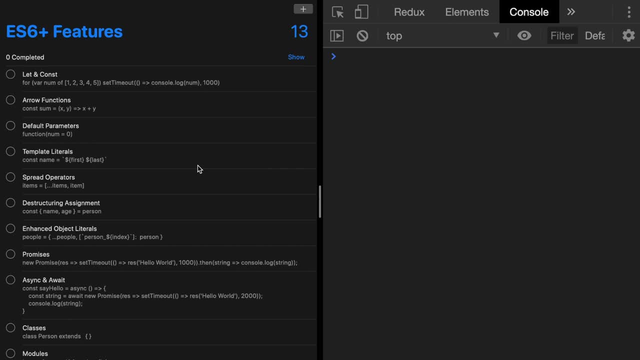 use most often. If you're wanting to use some kind of JavaScript framework, most of these are necessary. I'm really excited for this tutorial. A lot of these features have helped me out tremendously, so let's just jump into it. The first thing I want to cover are the let 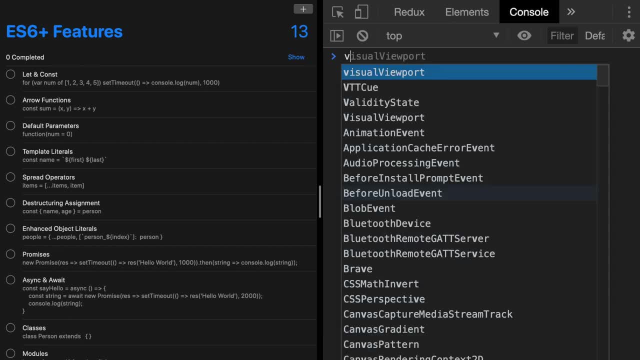 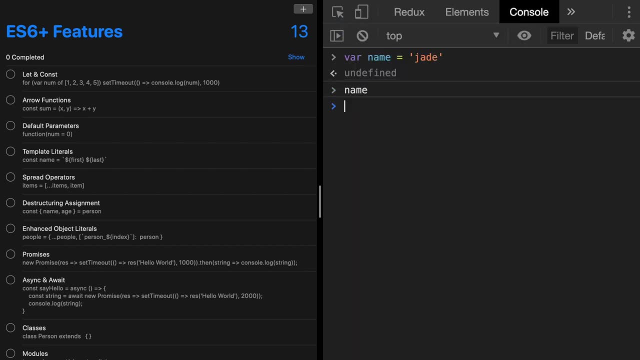 and const keywords. In the past we used the var keyword And since it's a var, we can reassign it. But now you're going to want to use the let keyword And if it's a let, you can still reassign it. 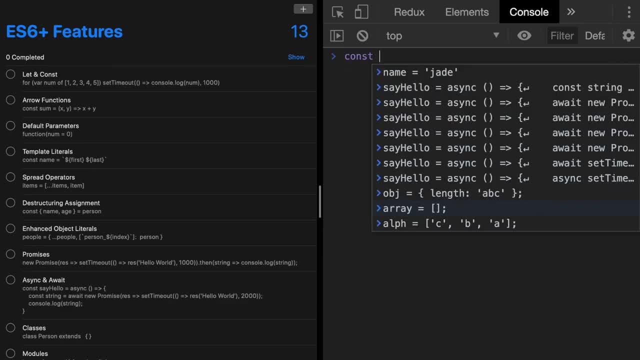 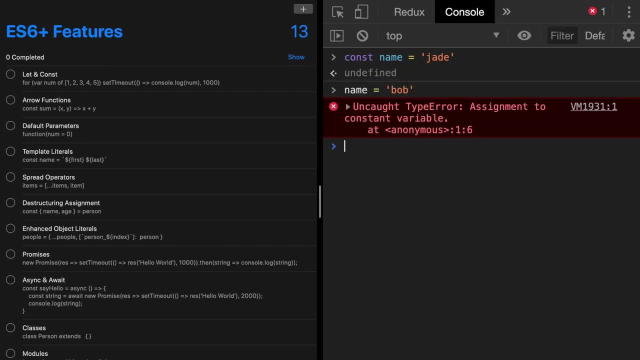 But if you make it a const, you can't reassign it. You can see how this will be useful if you have a variable that you don't want the value to be changed. This works with objects as well, So since it's an object, I can update the name key. 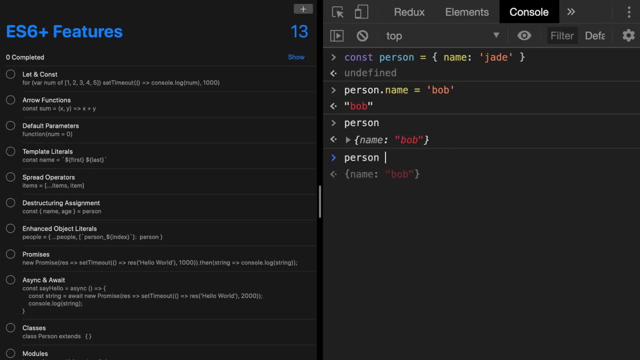 But I can't assign that variable to a new object And that's because objects are assigned by reference. Let me show you what I mean. So if I made another person and I updated the name of the first person, the name of the second person also updates. 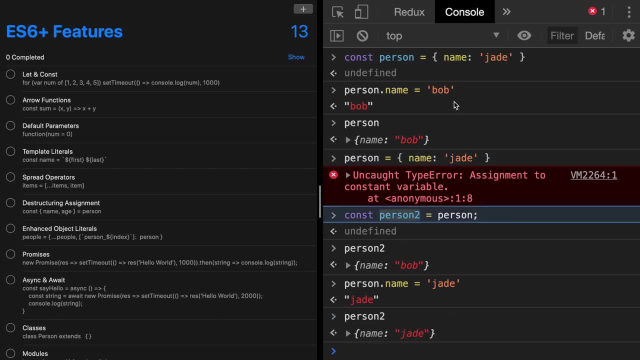 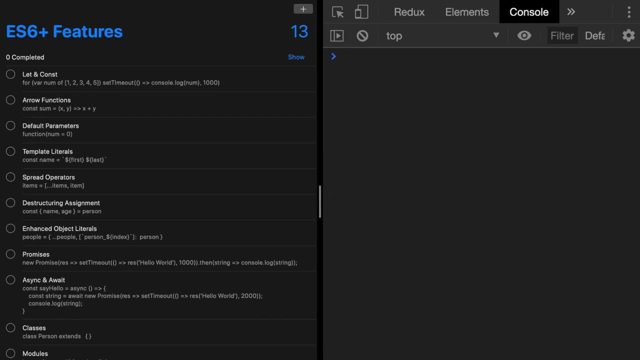 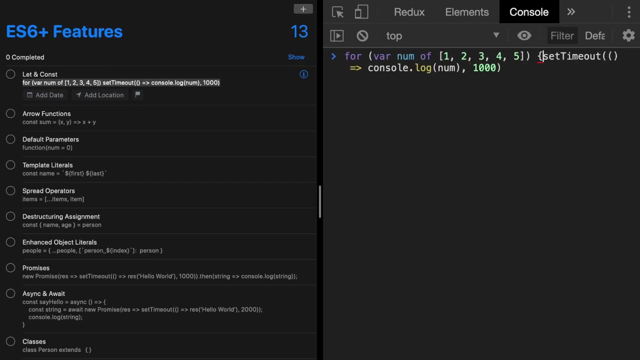 That's because person and person2 are referencing to the same object. Also, I've seen this problem in interviews before. Say you have a for loop? I actually have the example right here. I'll just format this a little bit. We get five, fives. 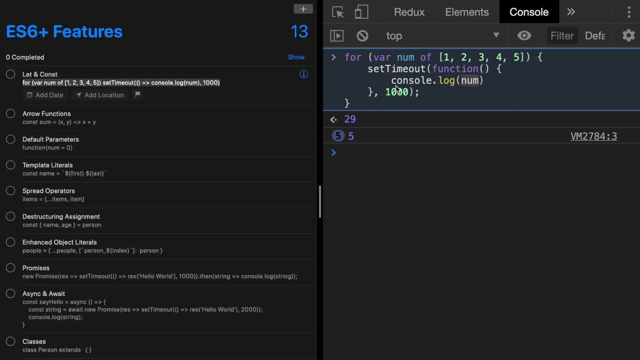 And that's because person1 and person2 are referencing to the same object, And that's because num gets reassigned every time this loops. If we turn this to a let or a const, we'd get the result that we'd expect. Let me show you another example. 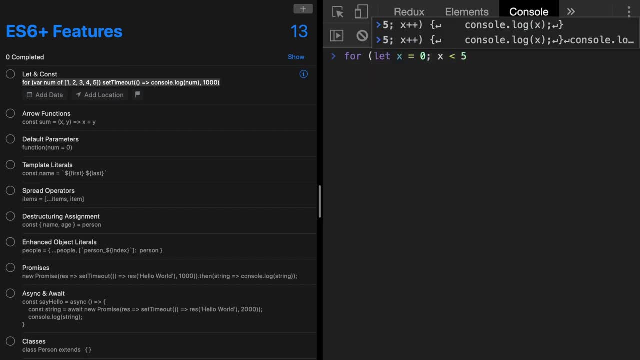 So if I run a for loop- Actually let me turn this to a var- So if I execute this, we get zero through four. Now if I just cancel out the x, you'll see that x is available outside of this scope now. 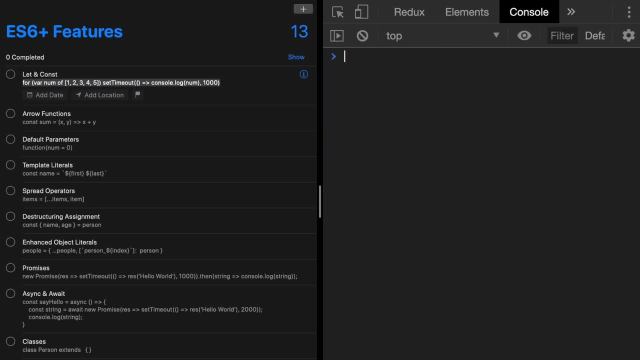 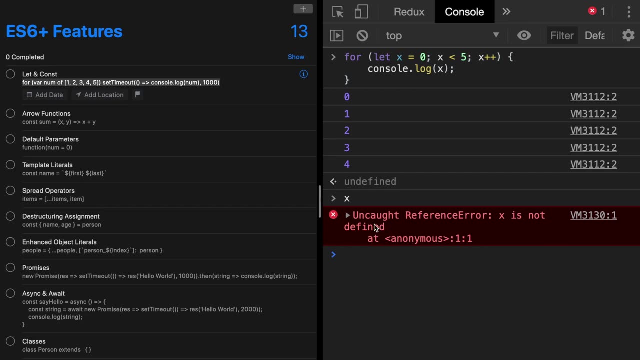 And if I used a let or a const, x is not defined. That's because x is only available outside of this scope, It's only available within this block. So try to use let and const instead of the var keyword from now on. 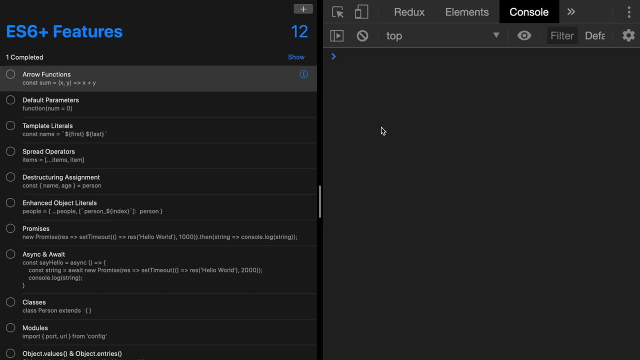 Okay, arrow functions- These are awesome. So if we want to write a function to return the sum of two values, we could write it like this: And then we could use it. And then we could use it, And then we could use it. 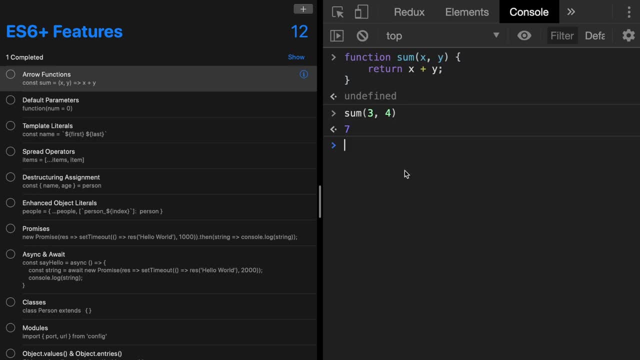 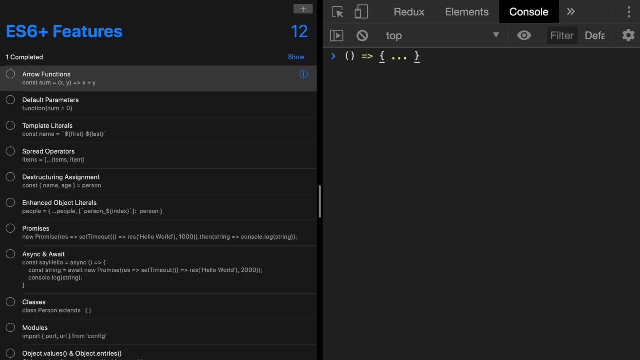 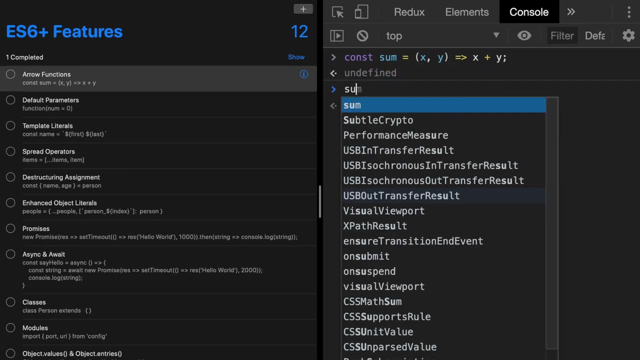 then your logic goes within here. We can assign it to a variable and use it the exact same way. We could also write it like this and save a couple lines of code, And that does the same exact thing. And if there's only one argument being, 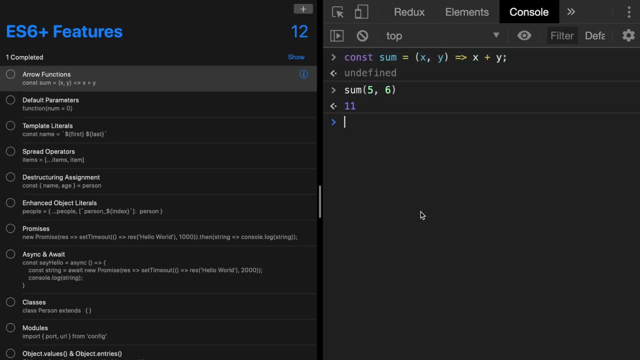 passed. you don't even need these parentheses. So maybe we make a function called add10.. And now we can just add 10 to any number. But not only do these read and write better, they also handle the this keyword differently. So this is actually just a counsel for this page. right here We went over this. 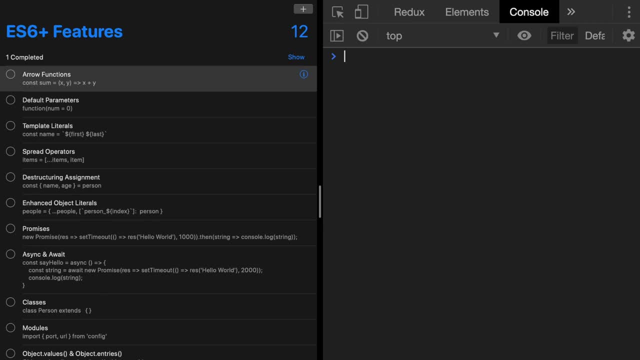 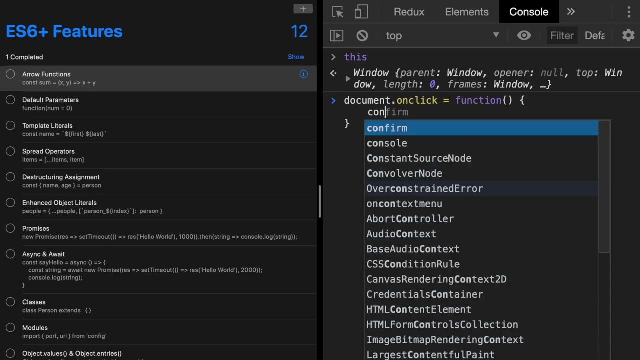 in the advanced JavaScript tutorial. If I just counsel out this, you'll see that this refers to the window. Now let's say I add an event listener to the document Inside. we'll just counsel out this And if we click on the document, 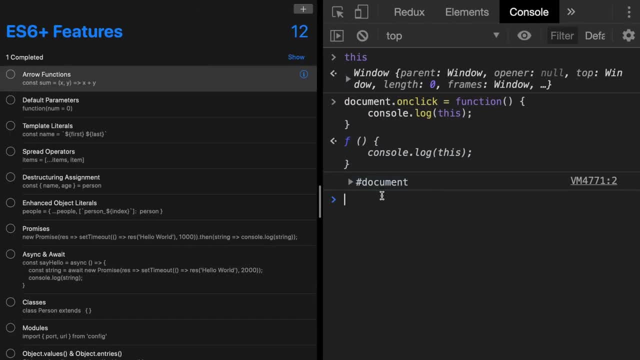 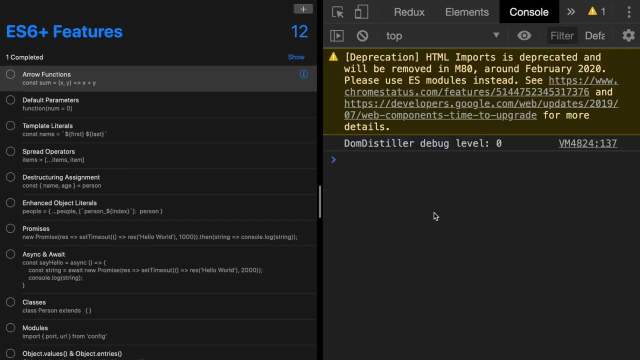 we'll see that the event listener has been added to the document And if we click on the document, we'll see that the event listener has been added to the document And if we click on the document, this refers to the document, compared to if we use an arrow function, which will 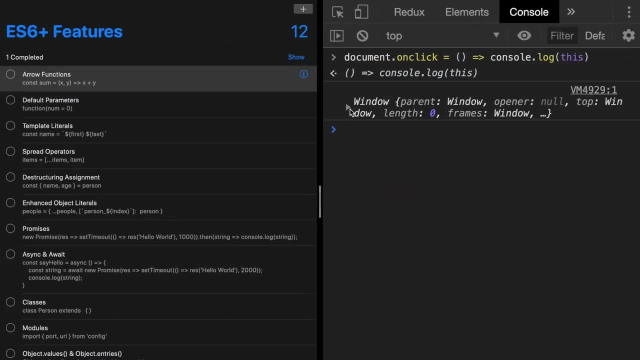 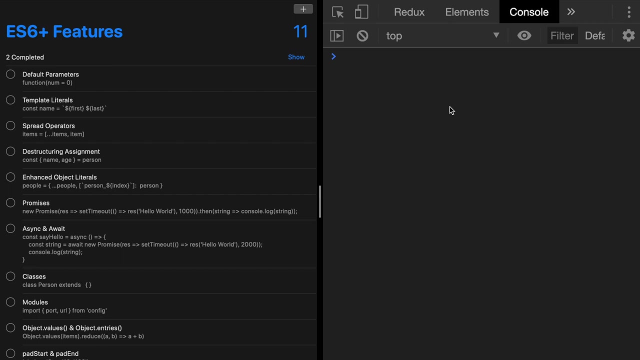 return the window to us. It will become more apparent how useful arrow functions are when you start working with classes and other JavaScript frameworks. Another really cool feature is you can add default parameters now. So let's say we wanted to add some default parameters to our sum function. Now I can call the sum function. 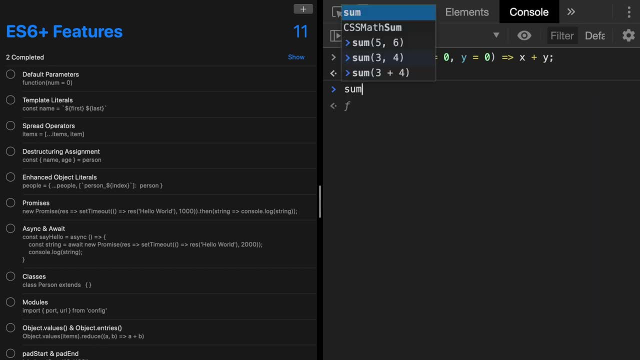 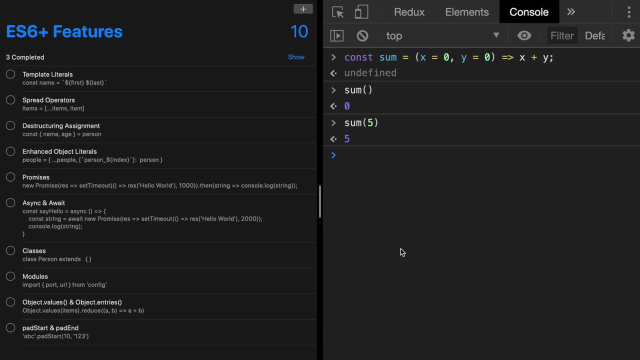 without even passing it anything, Or I can just pass it one thing: A super useful feature. Template literals are probably one of my favorite new features. Let me show you how this works. Let's create a function that says hello. Now, we used to have to concatenate it like this. 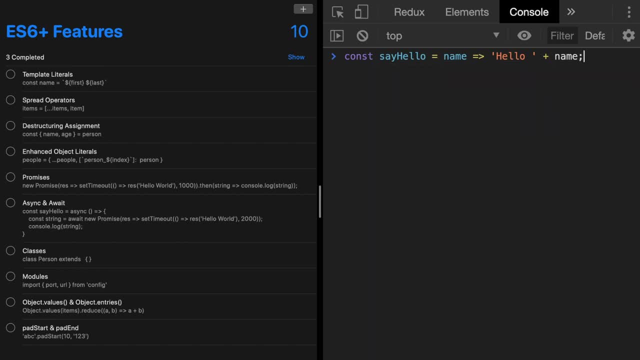 which has always been a pretty big pain, especially if you have a bunch of variables that you want to concatenate into a string. But they've made it super simple with template literals. You just have to use a back tick And then you can say hello, and then dollar, sign, curly boys, and then 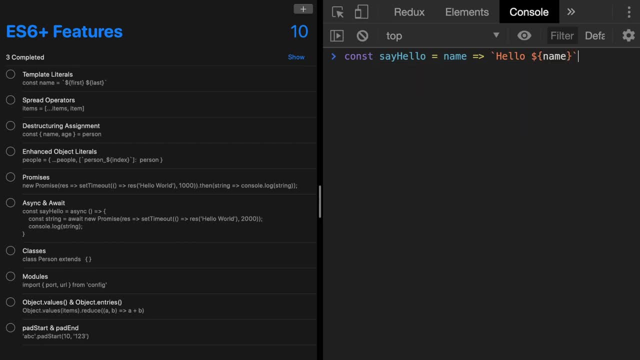 you put the name of the variable that you want. Isn't that awesome. Not only can you concatenate variables into a string, but you can also do multi-line strings now, And that's how that looks. What an awesome feature. I remember you used to have to do stuff. 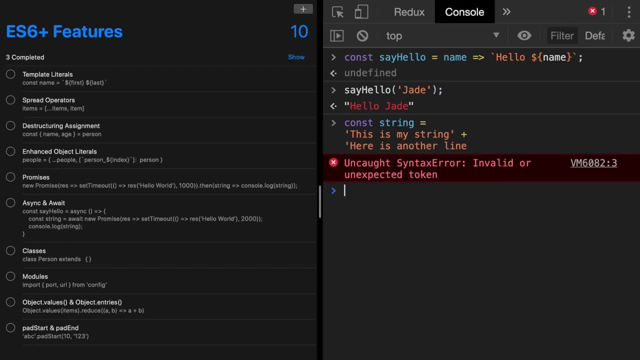 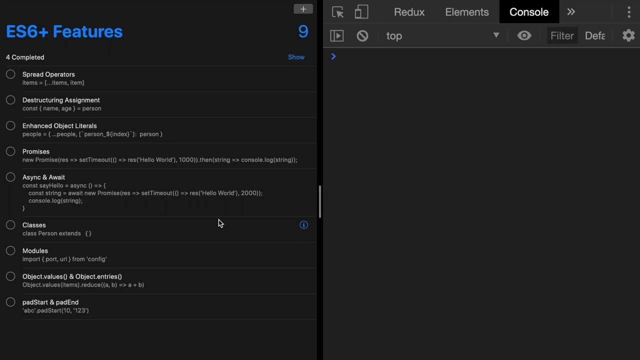 like this: Whoops, But you get the point. Now you can just put in a back tick and add as many lines as you want. One of my favorite features: The spread operator, makes it easy for us to copy over values from an array. Let's say we have array. 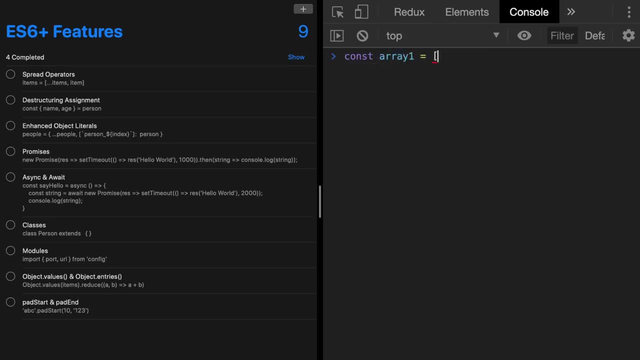 one And it has one, two, three, four, five, And we want to make array two And we want array two to have all of these values. but we want six, seven, eight, nine. We can do that like this Array two. 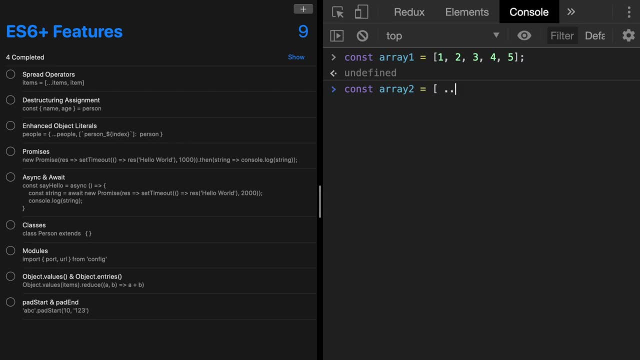 then we do dot, dot, dot, array one, and then we can just add the rest of the values that we want- six, seven, eight, nine- and you'll see that array two has all of those values now. or we could even do: array three equals six, seven, eight, nine, and we can say array 4 equals array 1, with array 2 or with. 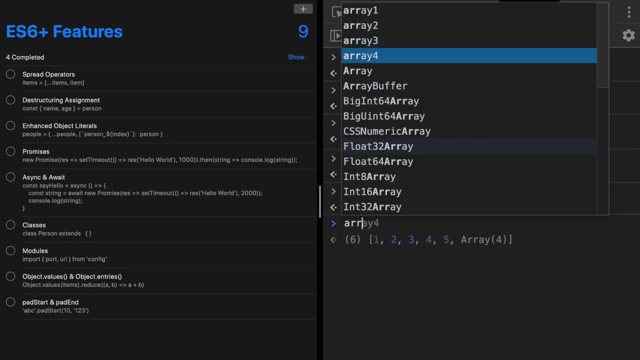 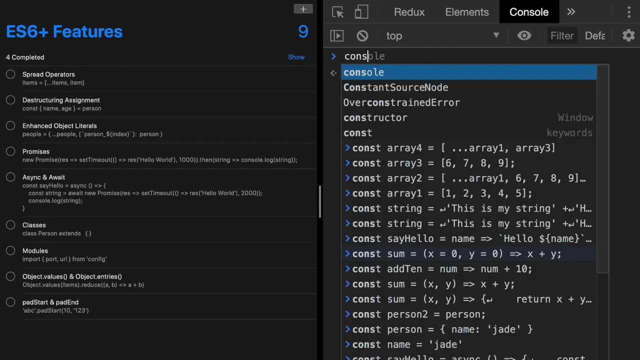 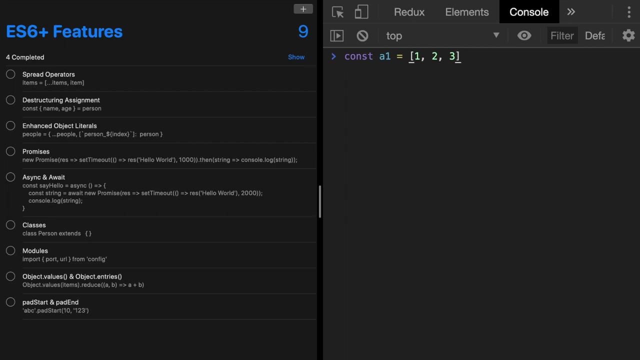 the right three. whoops, I just added that array in there. let me do that again, again. So array 1 is 1,, 2,, 3, and array 2 is 4,, 5,, 6, and then we can make array 3 a1. 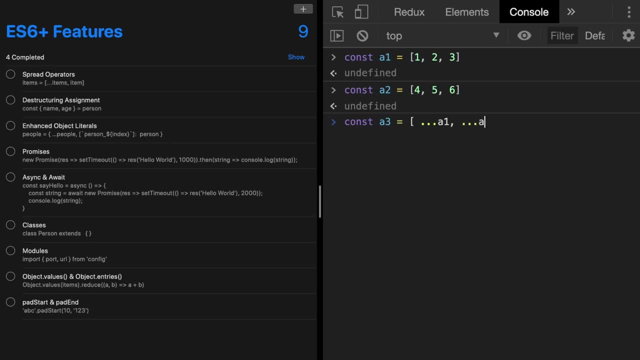 plus all the values in a2.. Not only can you use the spread operator with arrays, but you can use it with objects as well. So let's say we have a base person. Now we could create a new person and copy over all of those values at first. 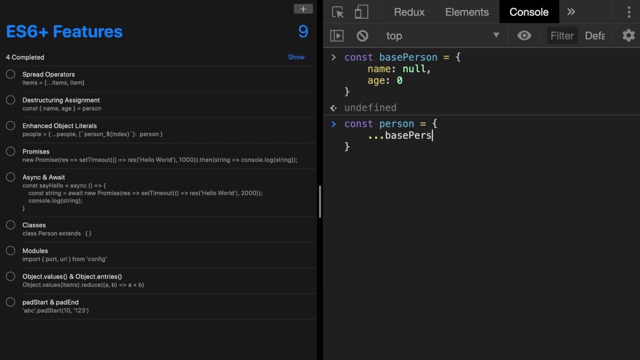 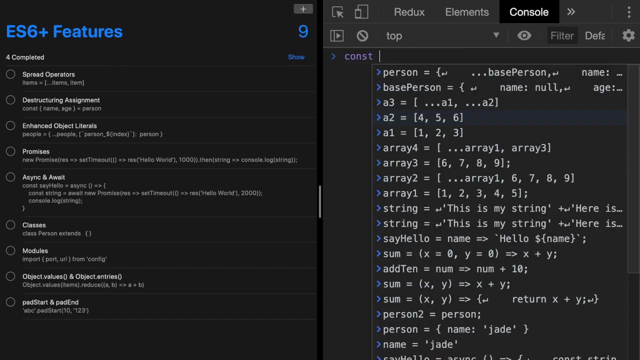 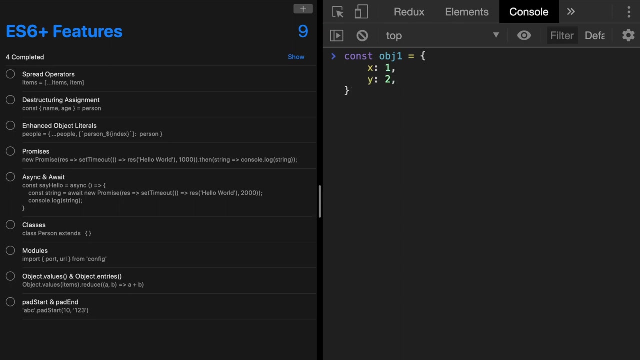 And then overwrite some of them. You can also add more keys to an object, So let's say we have object 1.. You can also have trailing commas now, So I could add a comma here and it wouldn't give me a syntax error. 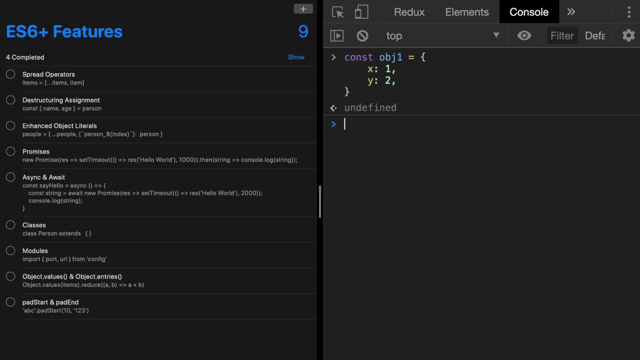 But something to keep in mind about arrays is it will still add a value at that index. So say, for instance, if I just created a new array with a bunch of commas in it, you'll see that it will create an array with the length of 5.. Anyway, let's make our object 2 now And let's try to 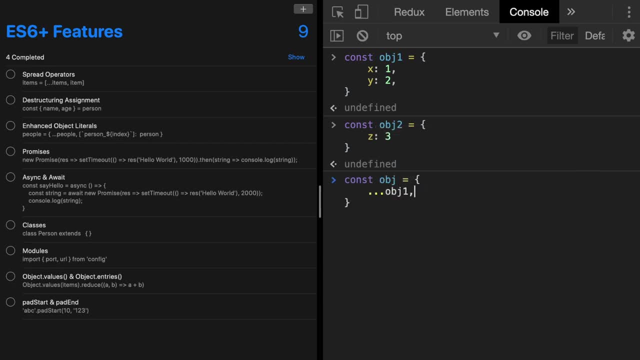 combine them and maybe do some other things. I hope that helps you understand a little bit more about how the spread operator works. You can also use it to create a new object from another object. Say for instance in our other example, where we made a Person object and then we made a new person from that Person object and we 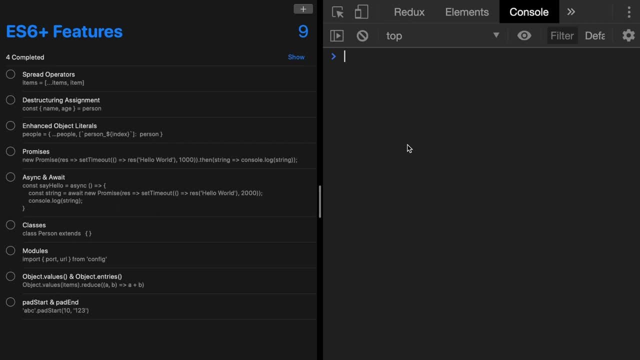 changed the name And, since it was created from reference, when I change the name of the first person, it changed the name in the second person, So let's reset that up Now. if I just made this equal person, that would be by reference, and if I change the name, 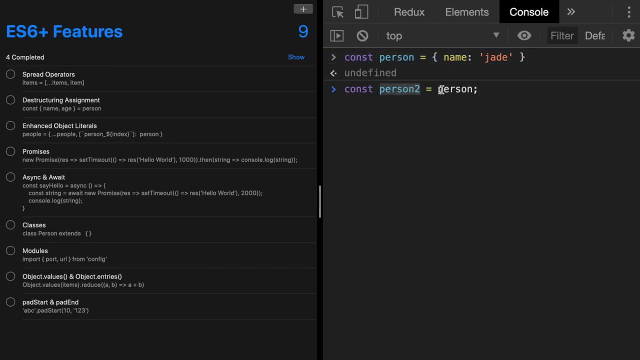 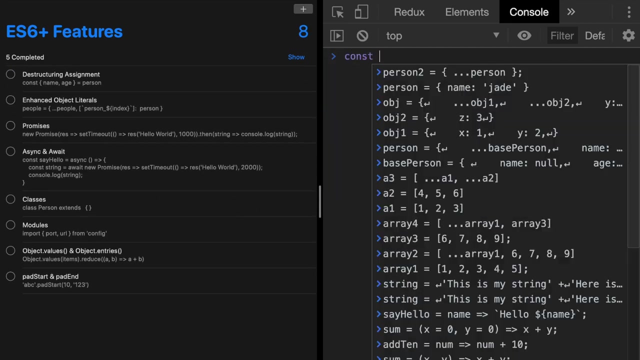 of person. it would also change the name of person too, but if we use the spread operator, it creates a whole new object. cool, so let's talk about you structuring. next, let's create our person again, and we want to do that in a different way. so let's do that in a different way. so let's do that. 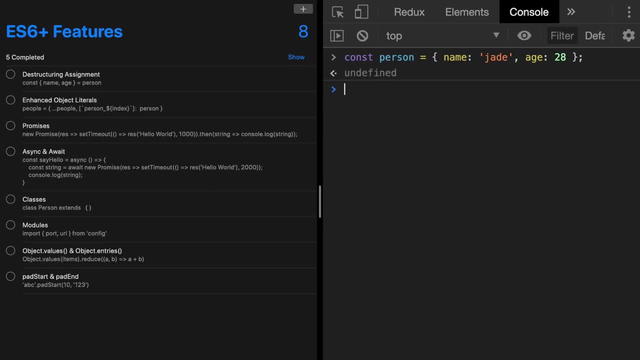 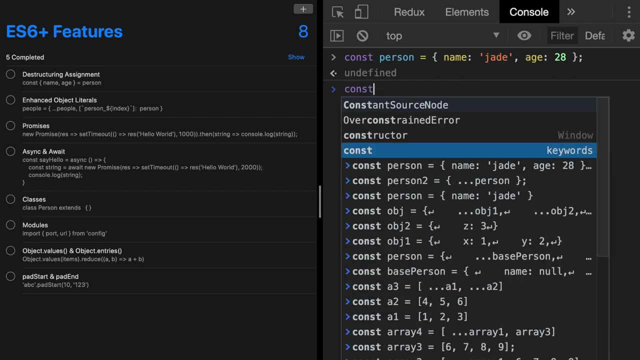 get the age out of this object. what we used to have to do is create a new variable, call it age, and make it equal to person age, and we'd have to do the same thing for name and so on. but now you can destructure an object like this: 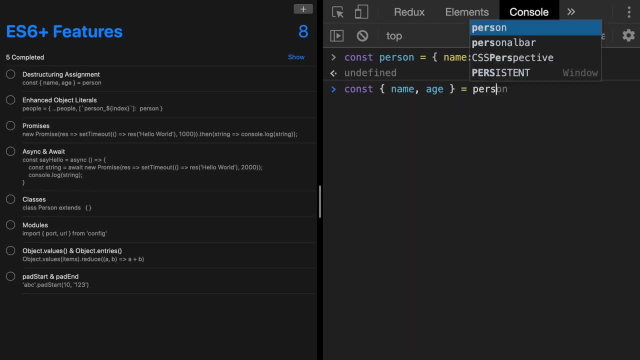 I can't tell you how useful this feature has been. this also makes it where we don't have to pass parameters in order anymore. let's create our function again to say hello. except for this time we're gonna pass it a couple parameters, we'll pass it the name and we'll pass it time of day. 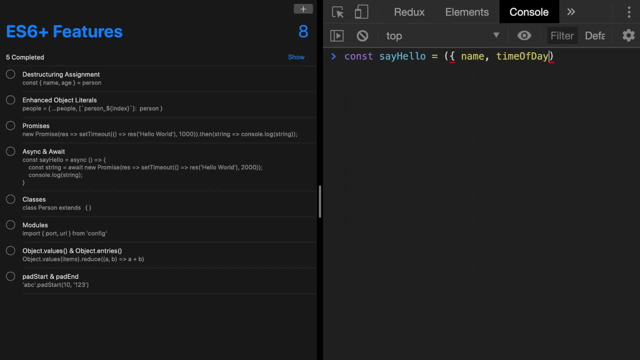 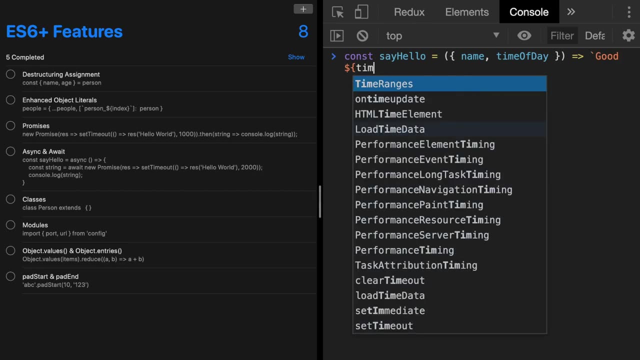 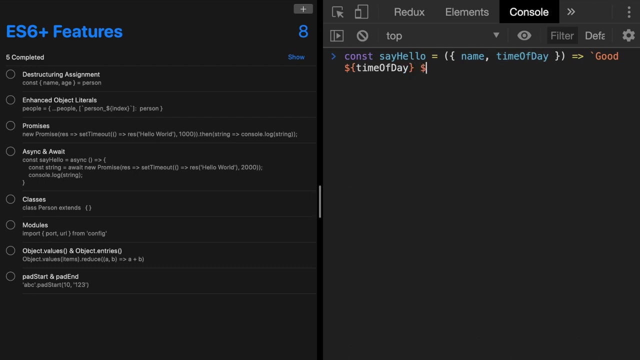 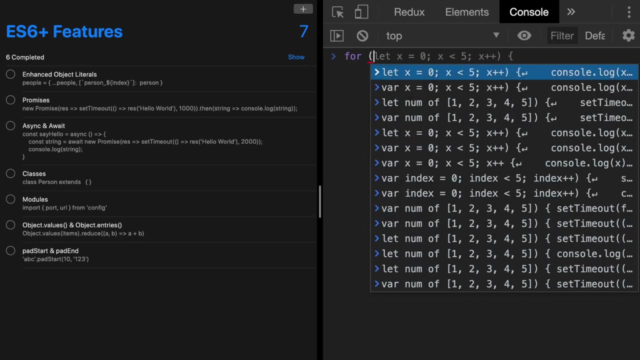 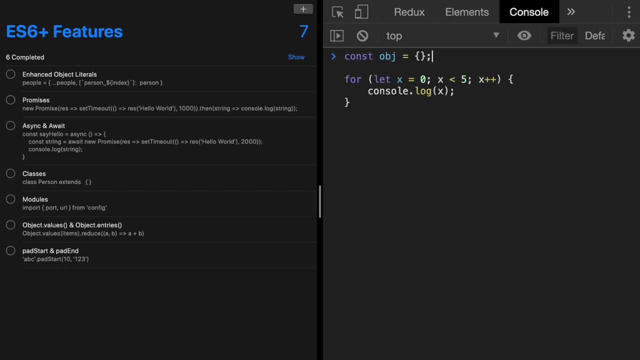 and we'll say: good time, time of day, whatever the name is. and now we could do something like this way, easier than trying to remember the order of all the arguments. we can also now add dynamic keys, so let me write a for loop again, but I'll make an object up here. I'll call it people. 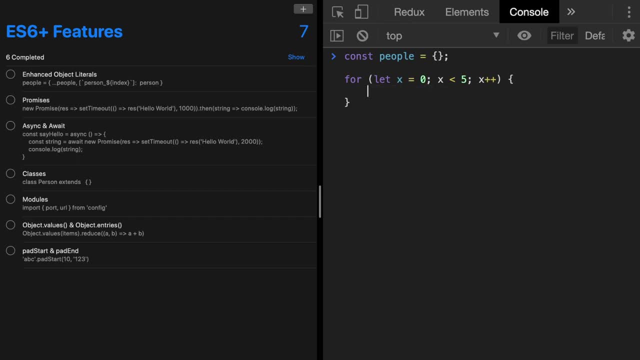 now I know I could just go people and then person X equals test X, but just for the sake of this example, let me show you how you would do it with the enhanced object literals. add all the people from before and I think that ought to work. I haven't used this one a lot, but it is useful to know. 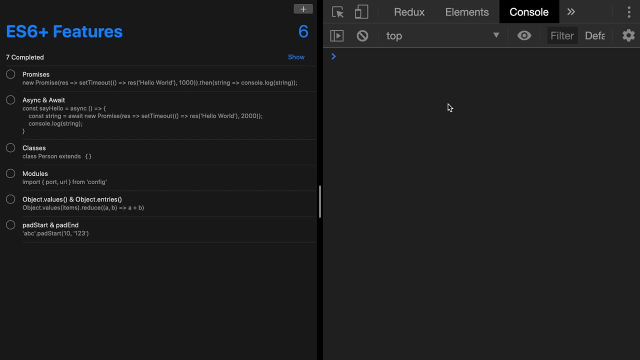 okay, promises- promises are awesome. let me show you how these work. so you just have to create a new promise. new promise and a promise takes a function, and this function has two arguments: a resolved and a rejected. so let's say we had a set timeout in here. 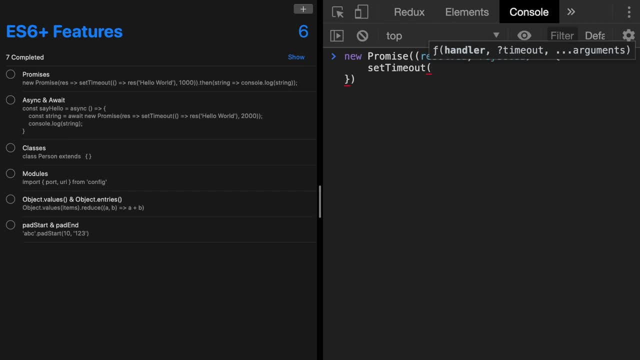 and in our set timeout we'll resolve a string and we'll set the timeout for like three seconds. now we can chain on a then statement and we'll get that string back and we'll counsel it out. so this function is gonna fire and this part is not going to execute until this has been resolved. 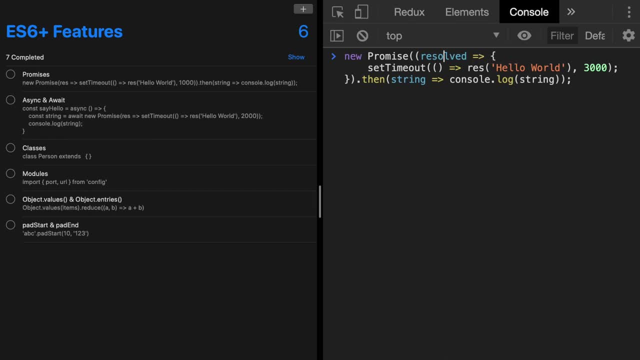 we don't even use rejected in this example, so we can just get rid of it, whoops. and I don't even use the word resolved. I use our yes. you'll see a lot of people use our yes for resolved and rejected, so so when I execute this, we shouldn't get any. 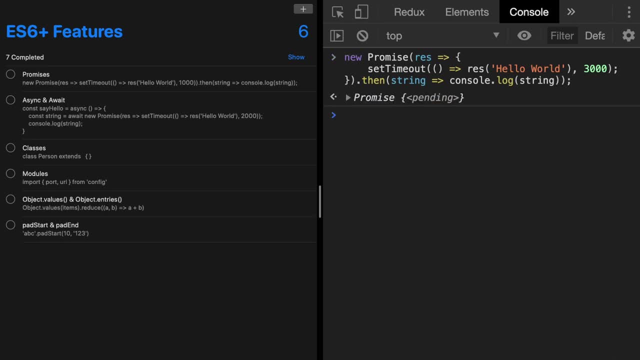 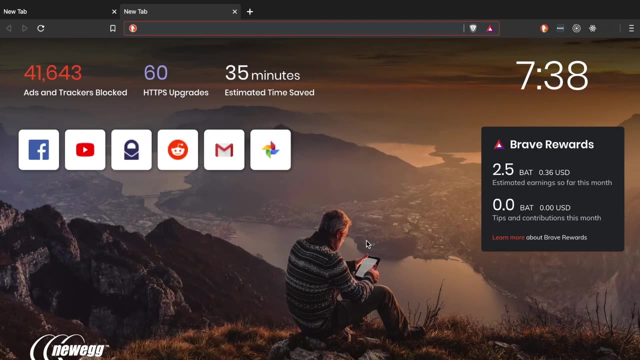 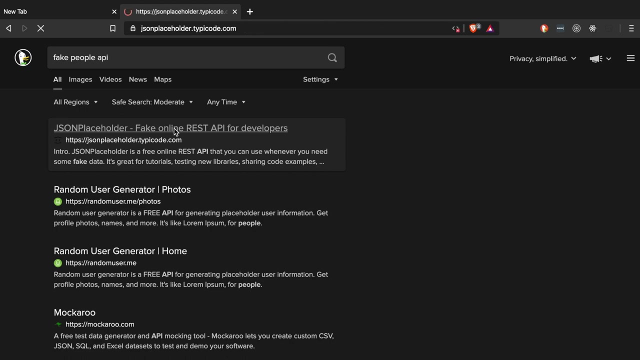 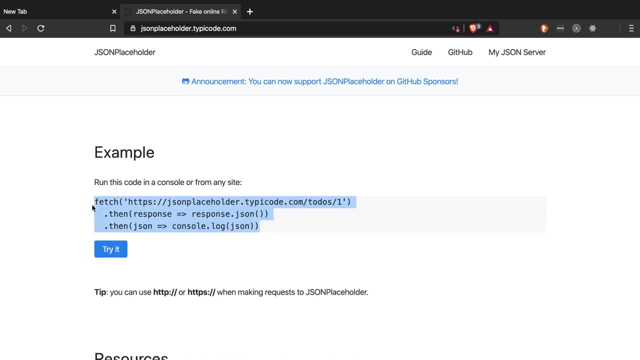 thing for three seconds. this is really useful when you start working with api's. so there's actually this fake API we can use for this example- fake people API- and here's this little example right here. so if I run this, it will go out and it's going to run the same thing over and over and over. 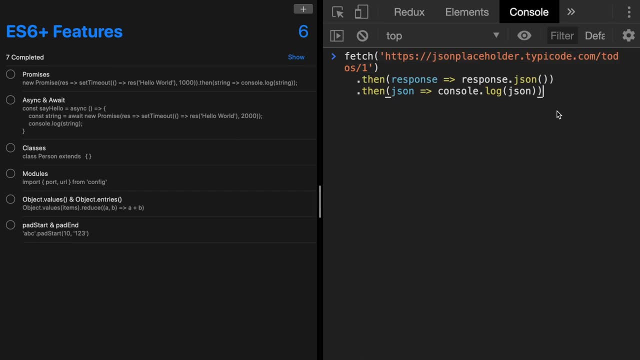 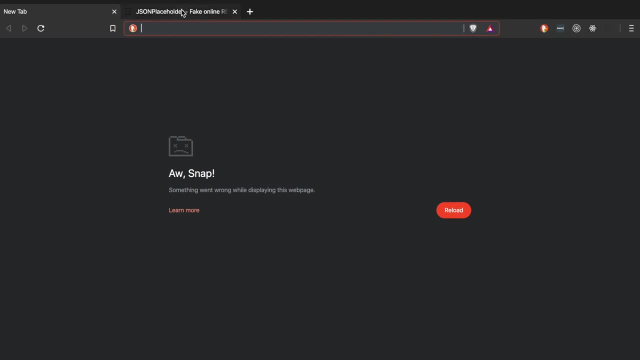 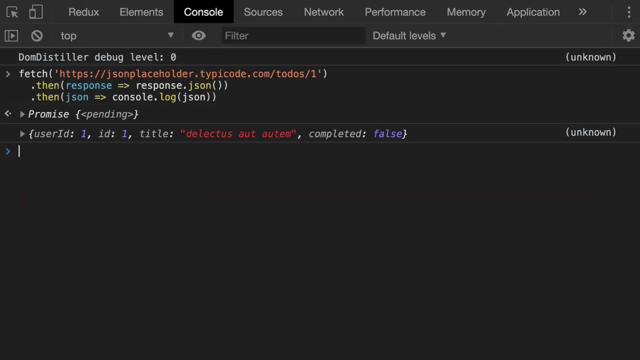 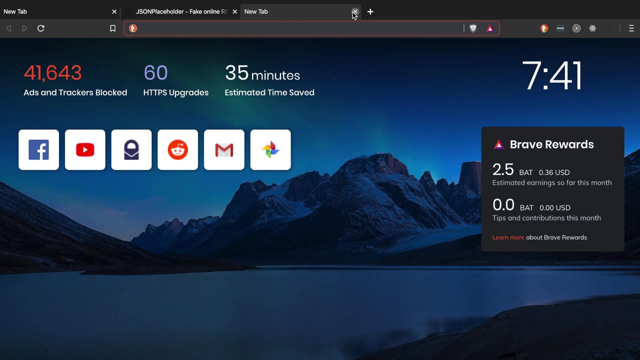 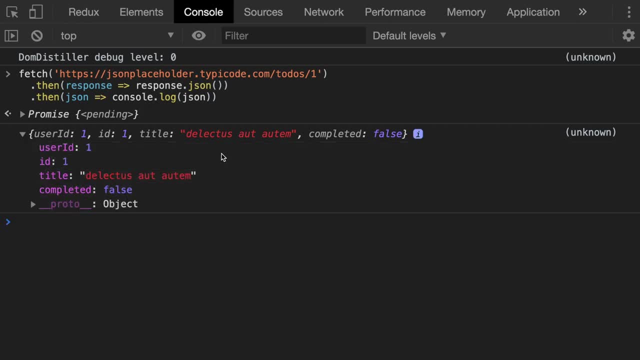 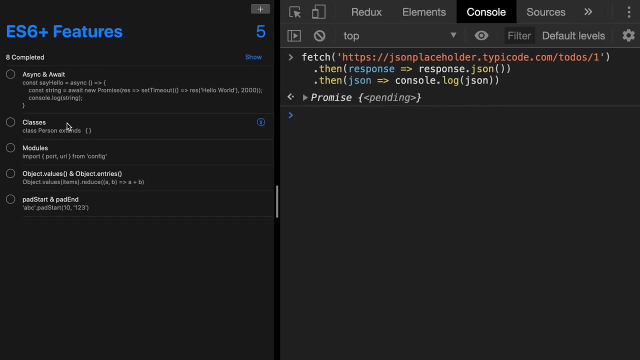 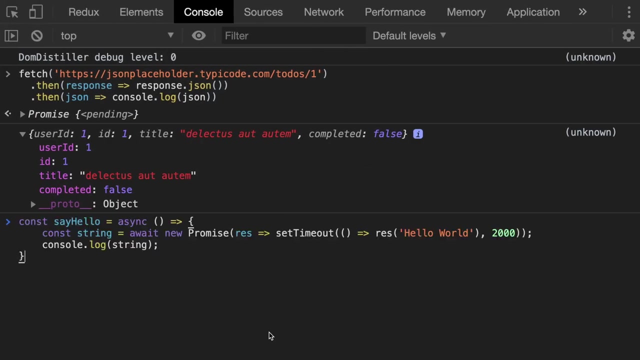 So you'll see that it returns this object. Now you'll also notice that fetch is promise-based. Fetch is a promise, and there's these, then, statements that are chained, which leads me to the next feature: async and await. Let's copy this example over and we'll 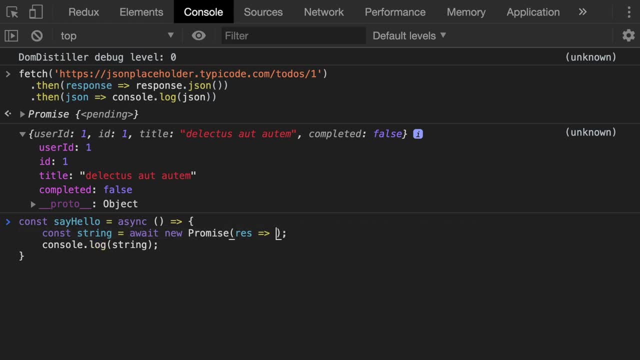 remove this setTimeout. We can insert this fetch request and then we'll resolve this with the title, And since we're fetching from this URL, we would probably want to add a new one. We could add a catch to this, just in case it fails. 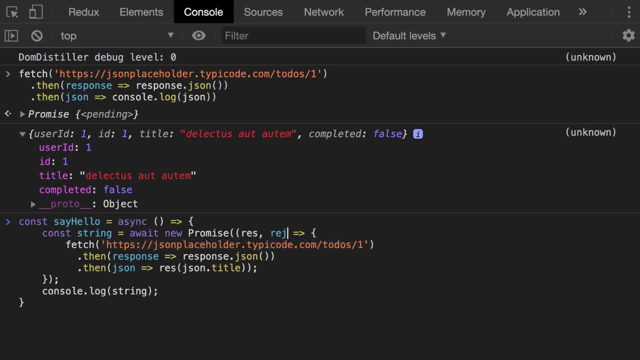 So we could add a resolve and we could add our rejected back. Then, if there's a failure, we can catch it And instead of say hello, we'll say printTitle. OK, let me go over this again, because it's. 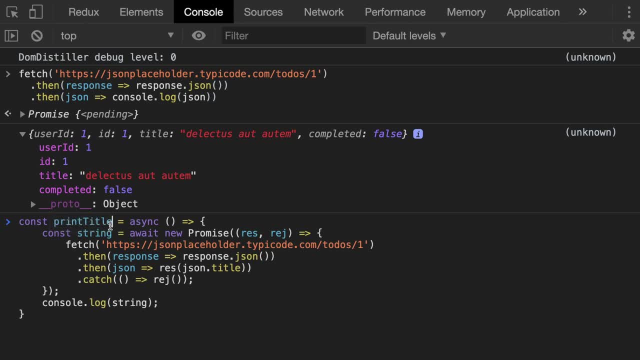 quite a bit of code. So we're creating a new variable which is equal to an arrow function, But this function is an async function. Now, if we make it an async function, we're able to use this await keyword within it. 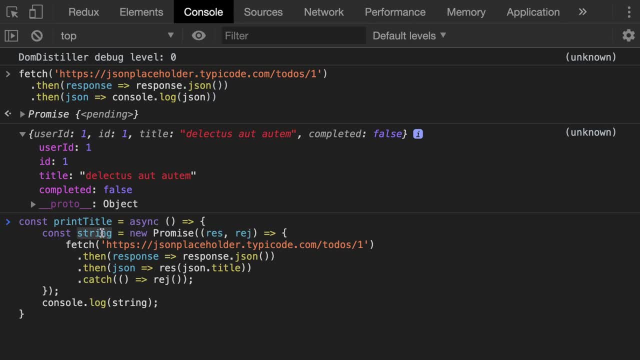 So if we didn't have this await keyword right here, this string would equal this promise and it wouldn't equal the value that's being resolved- OK, resolved. then it would just go to the next line and counsel out promise. but since we're using the await keyword, it's gonna wait until this promise is. 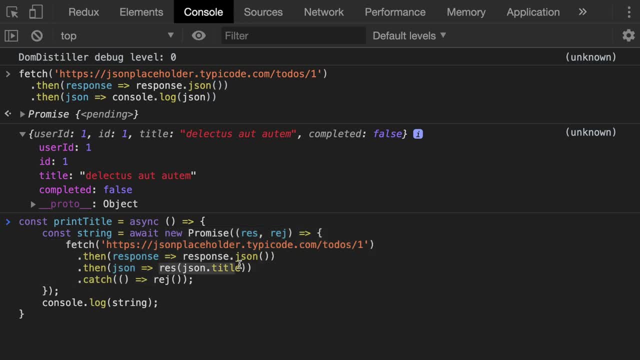 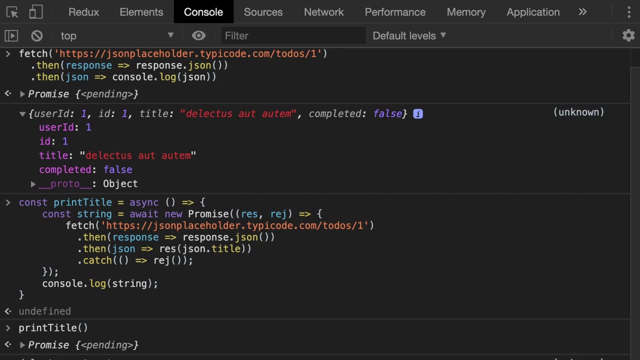 resolved and then it's gonna assign the value to the string and you'll see that we got the title right here. this becomes extremely useful when you start working with api's. for example, you could have a loading message show while your request is being processed. it also makes it way easier to write asynchronous code, as. 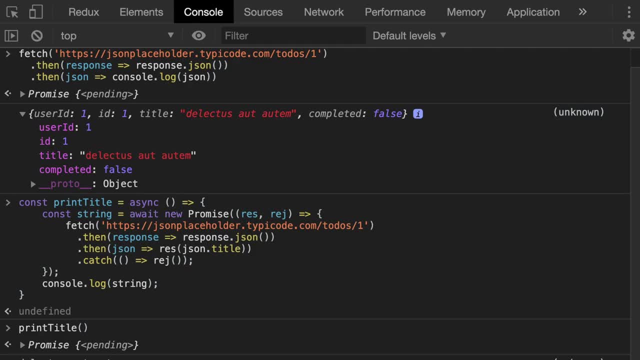 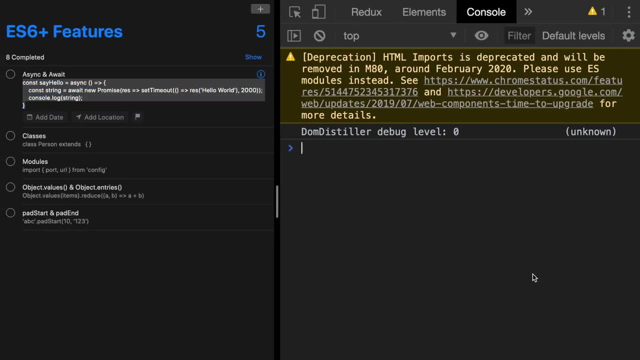 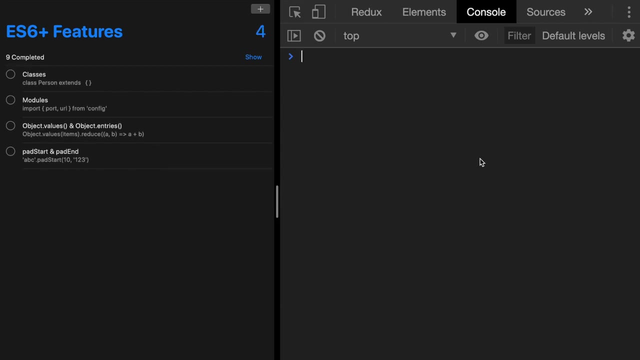 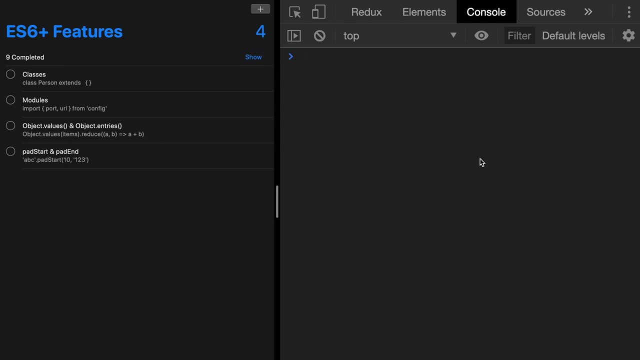 become the optimal solution. so let's create a class. we'll call it person, and every time you use this class to create a new person, a constructor is going to be called. so let's pass the constructor a name and we'll say this dot name equals name, and we could even add a default for this. 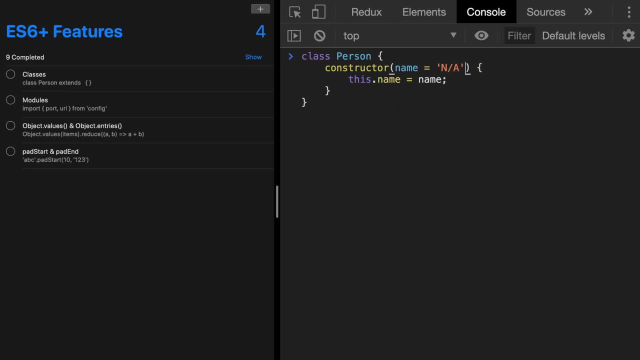 parameter. now we can create a new person. you'll see that it returns this object and we can pass it a parameter. we can also add methods to our class and we can give people a저on on a string. let's say, can create a new person and we'll say: 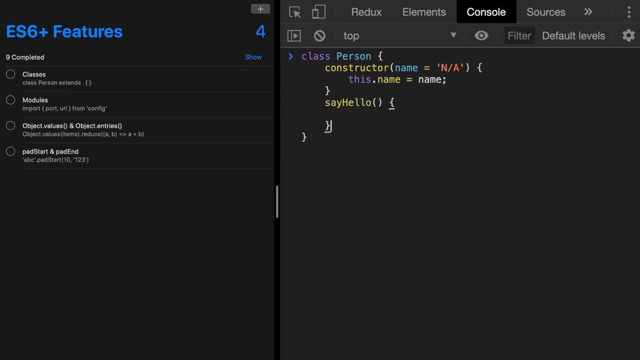 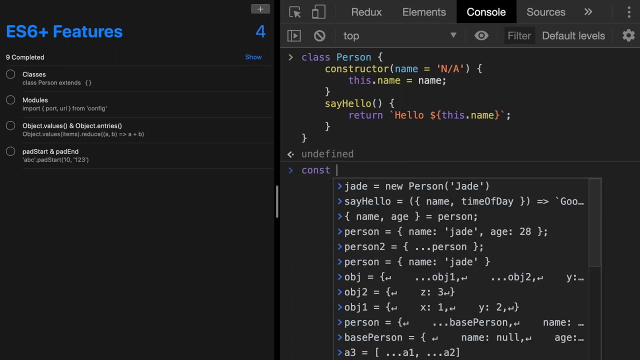 I'm going to save this for a moment. let's create another one for this class and reject. let's create another one for this class and reject. let's say say hello, this dot name, and we'll create a new person. we'll assign it to a variable and we'll say: 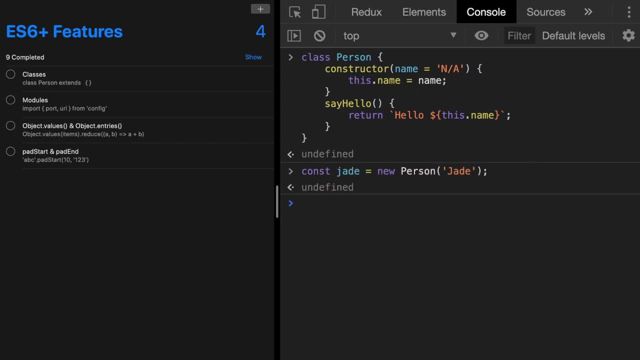 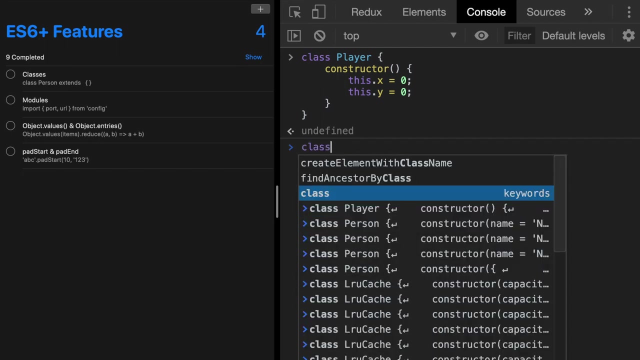 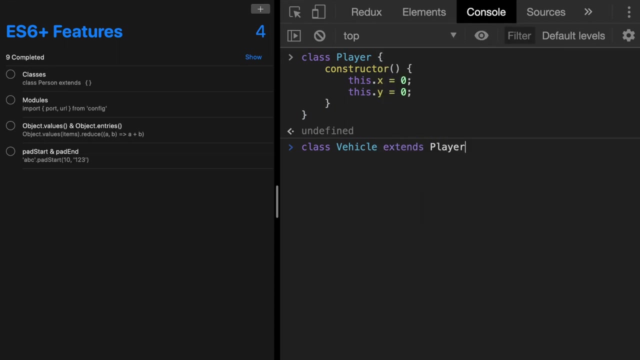 this dot name equals this dot name, slang one, and we'll flip over to the seventh type. say hello. You can also extend objects. Create a class called player, And we'll create another class. We'll call it. vehicle extends player, And since this is extending, 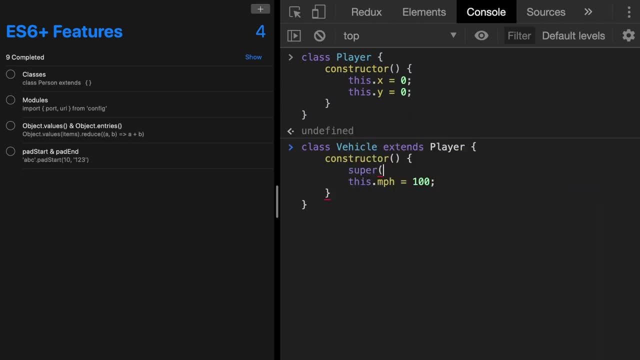 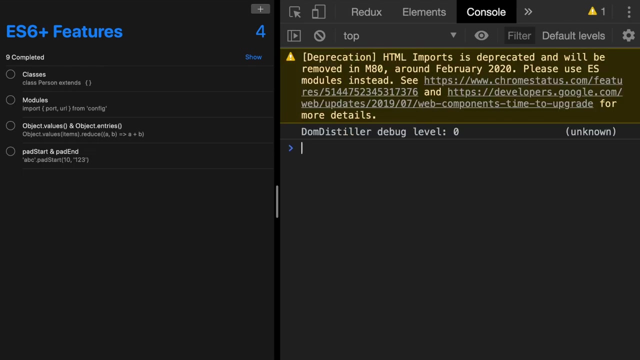 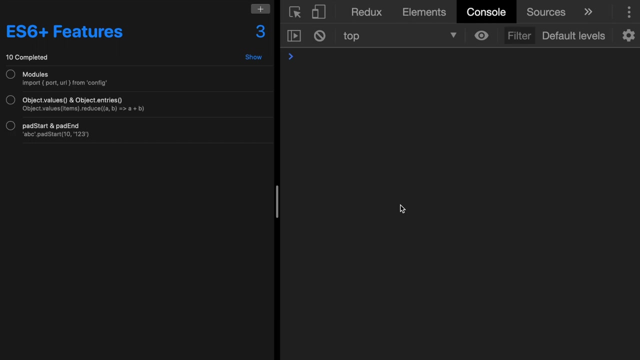 the player we're going to have to call super before. Kind of a bad example, but it gives you an idea of how you can use this. I won't be able to show you how modules work inside of my console, but I'll try to give you an idea. 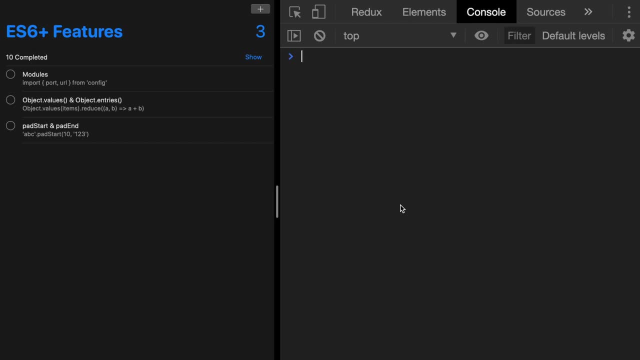 of where and how you would use them. So let's say, for instance, we have a JavaScript file called, Maybe, Let's say- settingsjs, And in settingsjs we have export const, port equals 880.. And we can export a URL. 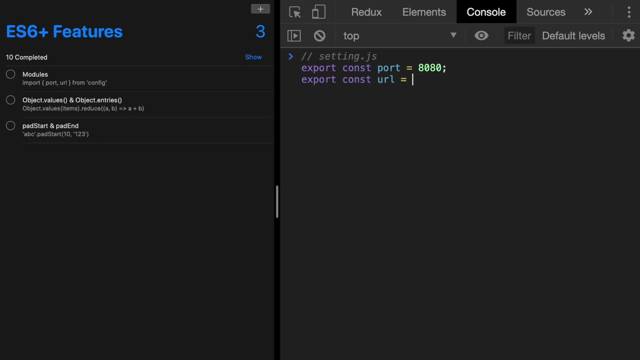 These don't necessarily have to be primitive values. This could be an object or it could even be a function. And then let's say you have another script called appjs, While inside appjs, at the very top of it, you can type import. You can import all as. 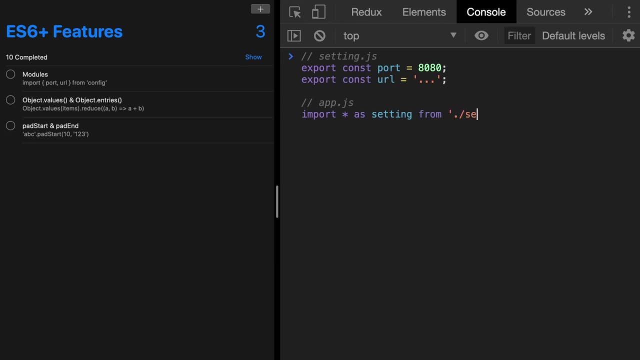 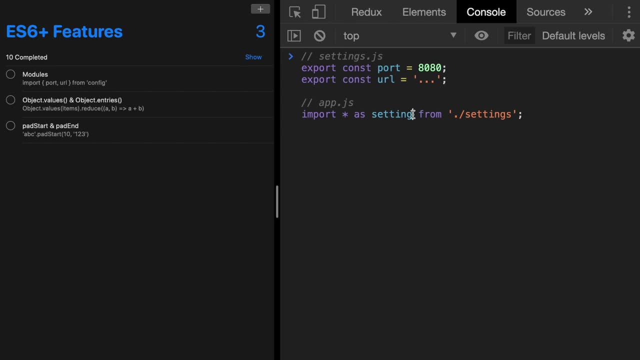 And then you can import all, And then you can import all, And you can import all, And then you can import all, And then you can import all. Or you can use the deconstructor, And then you're just going to import the port and the URL. 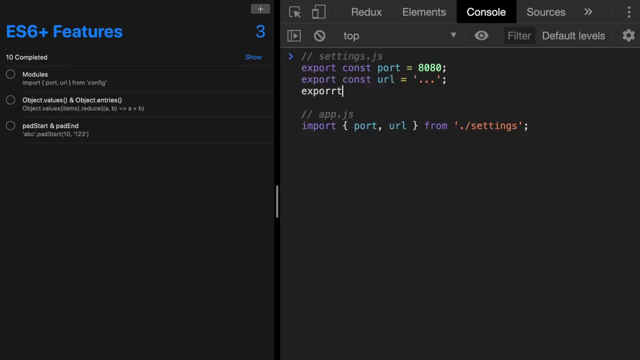 You also see things like this: export default. And that's so. you don't have to explicitly import all of these variables, It just defaults to this. So let's say we got rid of all of this, We don't need to do this. 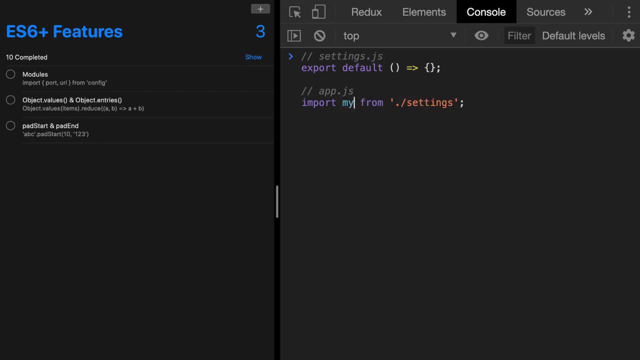 we can say: import my function from settings And it would be this function right here. We'll go more into depth about this feature in my React tutorial, And here's a couple other smaller features that are really useful. So let's create an object. 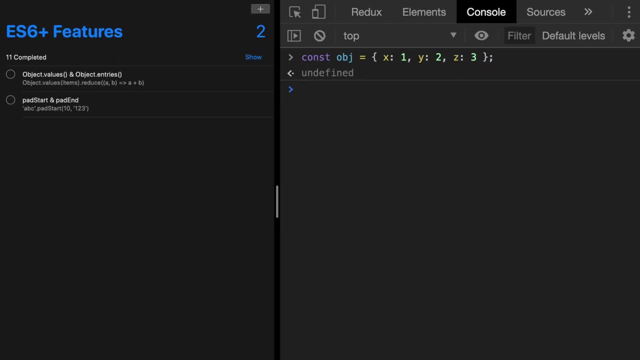 And we can get all of the values for all of the keys by doing objectvalues. And if we do objectentries we'll get an array of all the key value pairs. Last but not least, pad start and pad end. So if I have the string abc, I can say pad start.